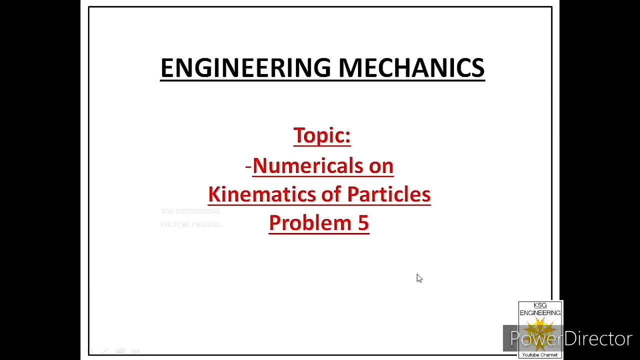 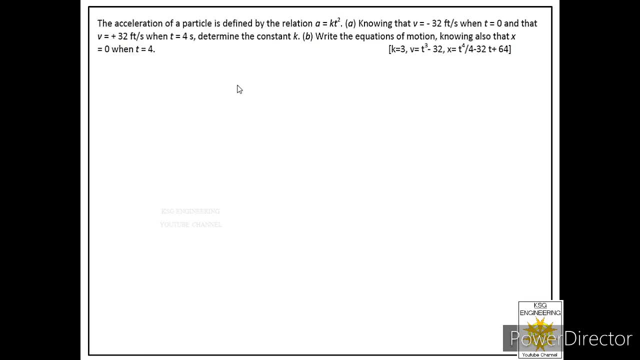 Welcome students. Today we will solve fifth problem on kinematics of particles. So let us start the lecture. So we are given one statement over here. Let us read that statement. The acceleration of a particle is defined by the relation a equal to kt square. 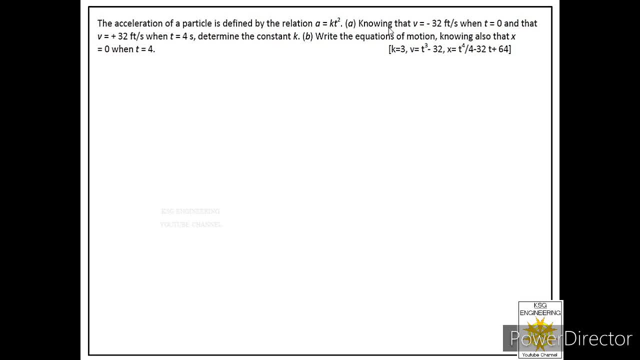 a part, knowing that v is minus 32 feet per second when t equal to 0 and that v equal to positive 32 feet per second when t equal to 4 seconds, Determine the constant k. So in this equation we have to find the value of k that is constant, and we are given two conditions. 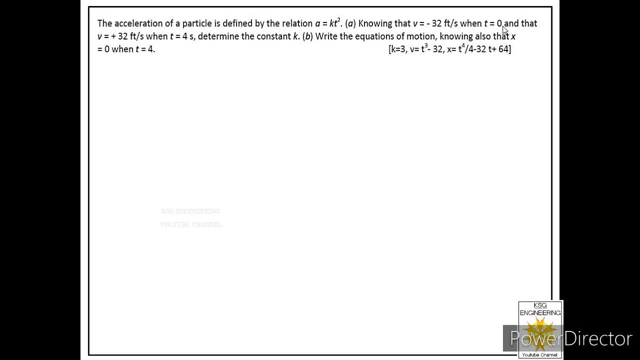 That we know that when time t equal to 0, the value of velocity is minus 32 feet per second, and when time t is 4 seconds, then value of velocity is positive 32 feet per second. Using these two known values, we have to find the value of constant k. 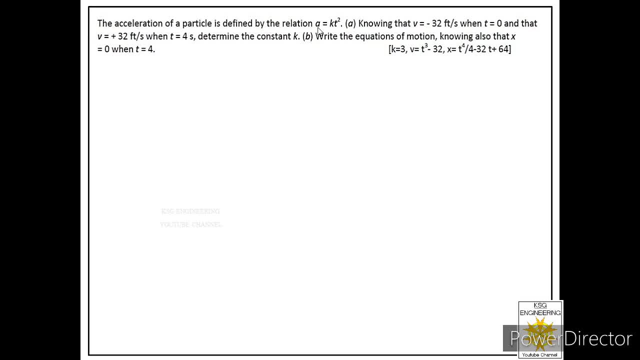 Now over here we are given equation of acceleration of the particle, which is in terms of t, and there is one constant, k also, And in a part we are given the values of velocity against the time. It means if we have to use these values, we first have to find equation of the velocity. 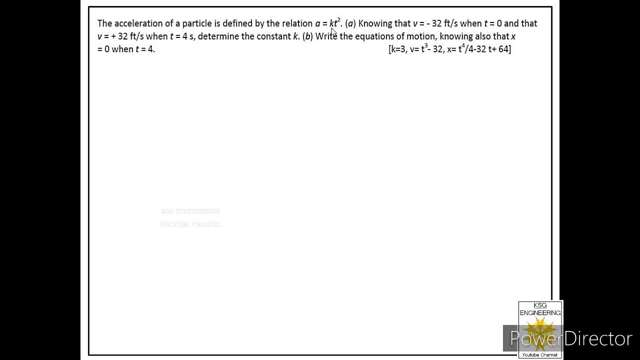 And we know, if we have equation of acceleration of a particle and we want to know the equation of velocity of the particle, then we have to do the integration of equation of acceleration of the particle. It means in this solution, the very first step is we have to take the integration of this equation. 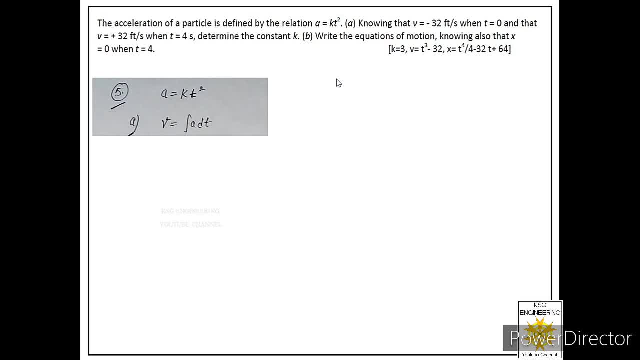 So let us solve a part. So we will say: velocity of the particle will be equal to integration of its acceleration with respect to time t. So we will replace a by this equation, that is, kt square, dt, and integration of kt square will be: 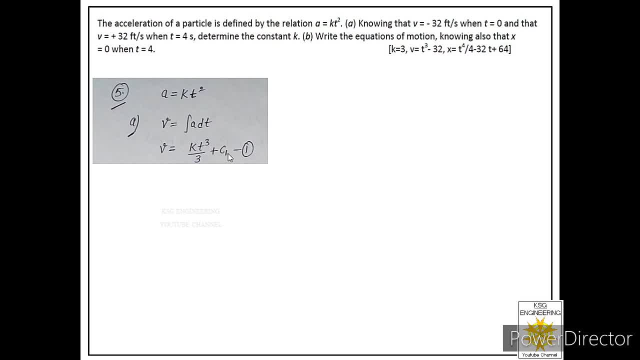 equal to kt cube by 3 plus. we have to add a constant over here. Let us say that constant is c1 and let us say this is equation number 1.. Now we will use these values given to us In the first part. he says: at t equal to 0, velocity of the particle is minus 32 feet per second. 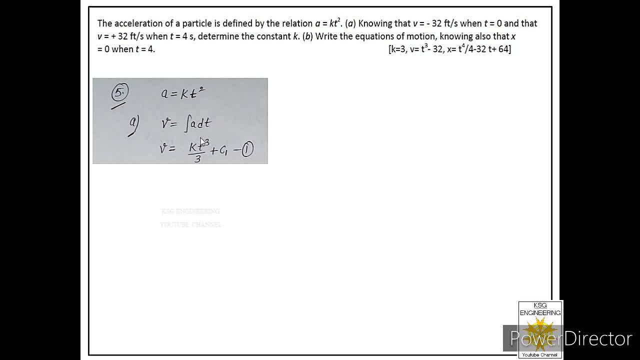 So let us put value of t equal to 0 and velocity as minus 32 feet per second. So when we put t equal to 0 and v equal to minus 32 in this equation, we will get value of the constant. So we have entered minus 32 over here. 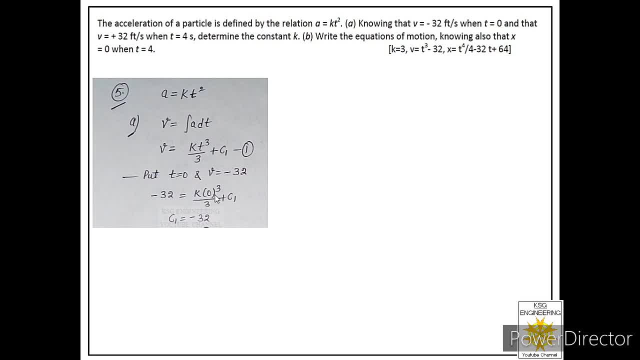 We have entered t equal to 0 over here and from this equation we will get value of t equal to 0. That is minus 32.. So we will say: put the value of this c1 in equation 1.. So that will be the complete equation of the velocity, because we have found the constant also. 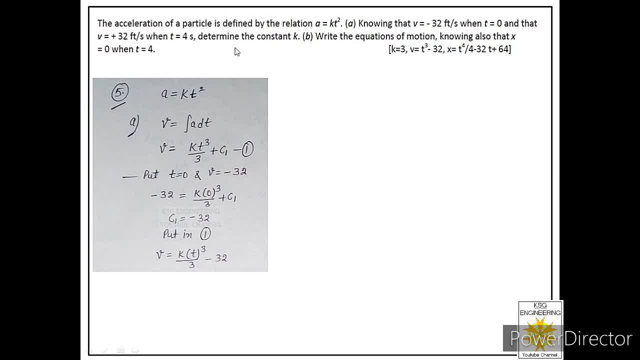 Now, after that, we will apply the second condition given to us, that when time equal to 4 seconds, velocity of the particle is 32 feet per second. So in this equation now we will put t equal to 4 and velocity equal to 32.. We can see over here: we have entered value of v as 32. 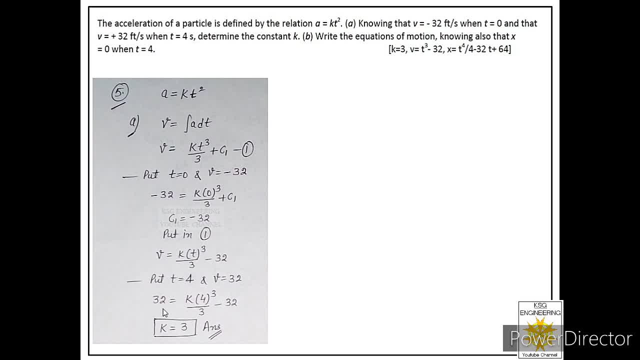 and we have entered value of t as 4.. So from this equation we will get the value of first part, that is a part that is the value of constant k equal to 3.. Now let us solve the b part. In the b part we are asked to write the equations of motion. 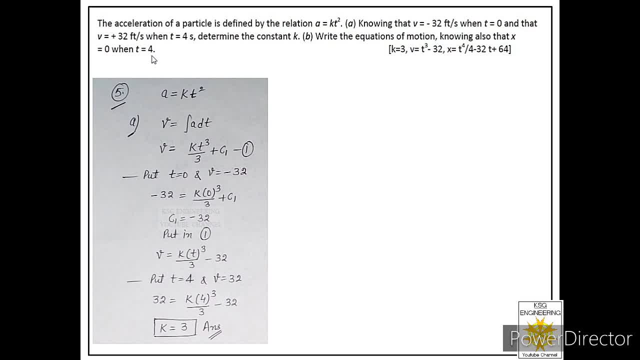 that x is equal to 4 and t is equal to 4 seconds. It means we have to write equation for the position of the particle and equation for velocity of the particle, And in the previous part- that is a part- we have found equation of the velocity. So let us write that equation. 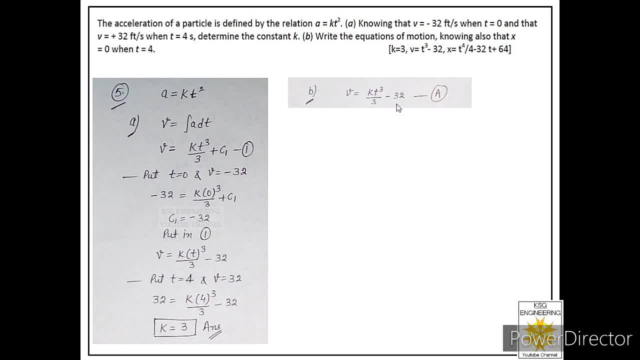 first, that is, v is equal to kt cube by 3 minus 32.. Now in this b part we are asked to find equations of motion. That means now we have to find equation of position of the particle and that we can find only after the integration of equation of the velocity of the particle. 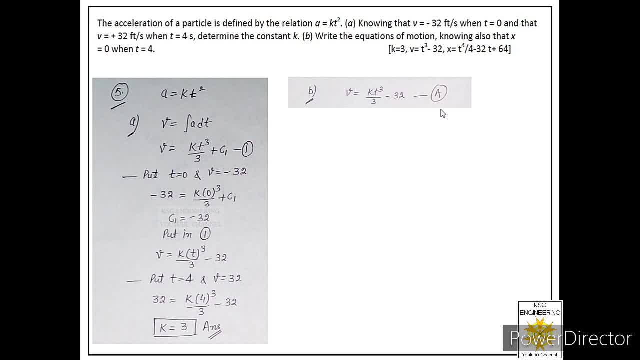 It means we have to do the integration of this equation to get the equation of position of particle. So that will be equal to x is equal to integration of v, velocity of the particle with respect to time. Now let us put the value of v over here and let us do the integration, So we will get kt 4 by 4 minus. 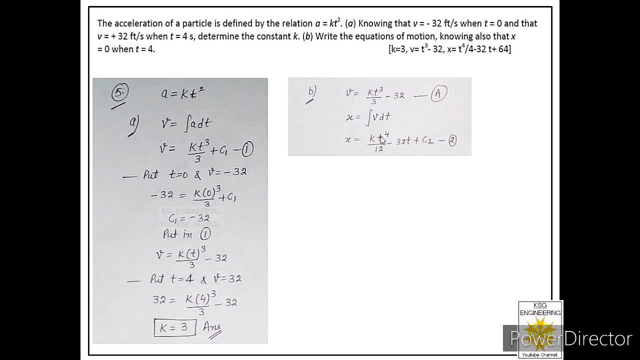 32t plus c2.. So we will write: x is equal to kt 4 by 12 minus 32t plus c2.. So let us call that equation as equation number 2.. So we have got constant over here. Now let us solve. 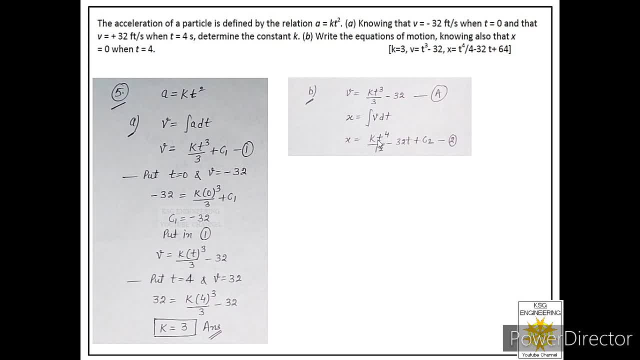 this equation. further Now, in this equation we know the value of k that we have already defined. So we have entered the value of k as 3 and we don't know value of c2. So let us find value of c2.. So how we can find the value of c2.. We can use this condition given. 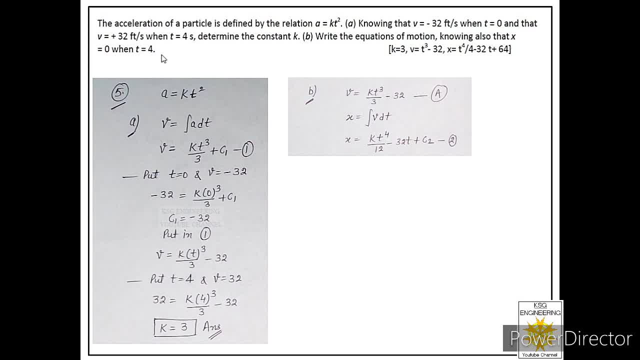 in the b part that x is equal to 0 when t is equal to 4.. So we will say: put k equal to 3, t equal to 4 and x is equal to 0 in equation number 2 and we will get value of. 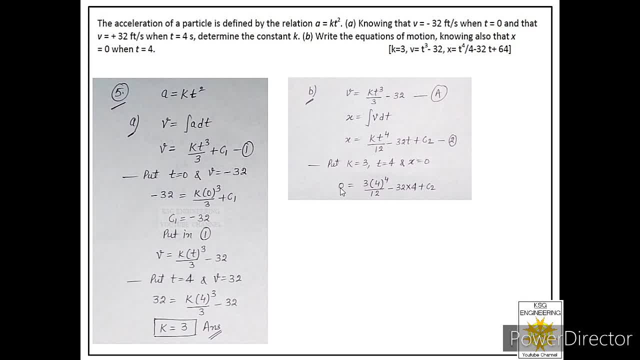 c2.. So we have entered: x is equal to 0. We have entered value of k as 3 and we have entered value of t as 4, and from this equation we will get value of the constant c2.. Now we will put this value in equation number 2.. So we will get equation of position of the. 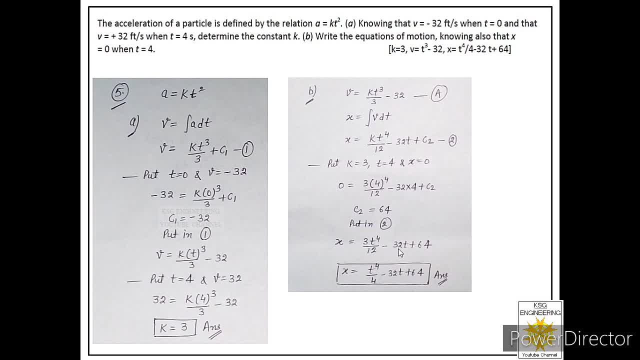 particle. So that will be 3t 4 by 12 minus 32t plus 64. And we will solve it further. It will become t 4 by 4 minus 32t plus 64. So this is the first answer. So we will write.